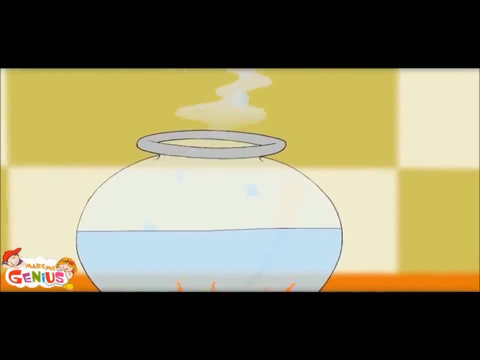 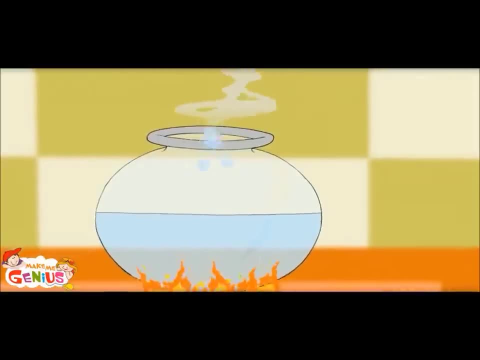 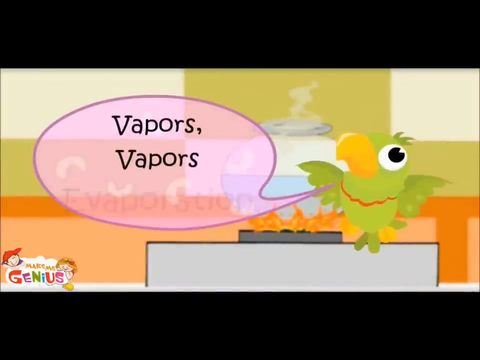 Some of them are coming out. We can see them, but they are forming a gas. So when vapor comes out of liquid on heating, it is called evaporation, Vapors, vapors, Evaporation. Now let me show you something. 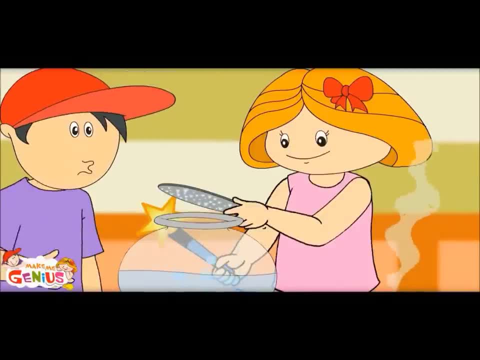 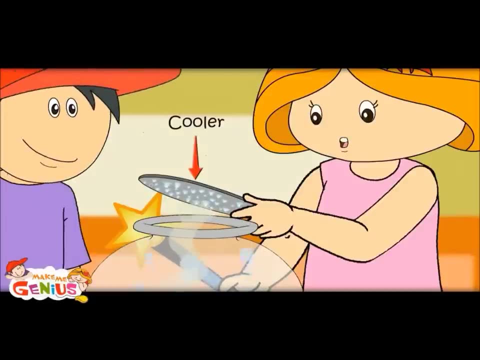 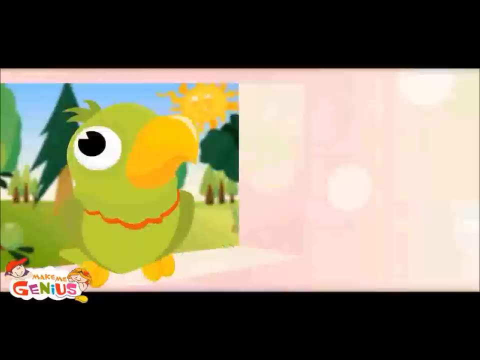 Oh, vapors are again becoming liquid. Yes, because the temperature of the cover is cooler than the temperature inside the pot, So molecules again start coming close to each other. This is how rain happens. When water vapors touch a cool surface, they become dense. 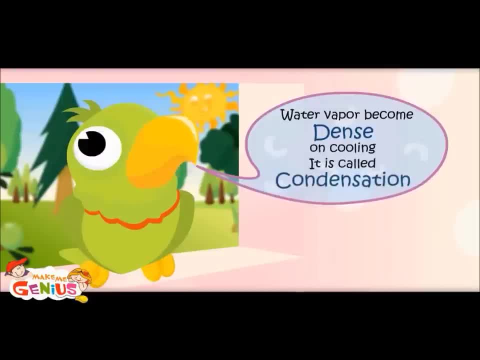 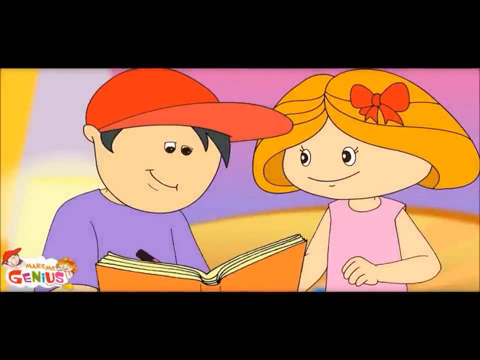 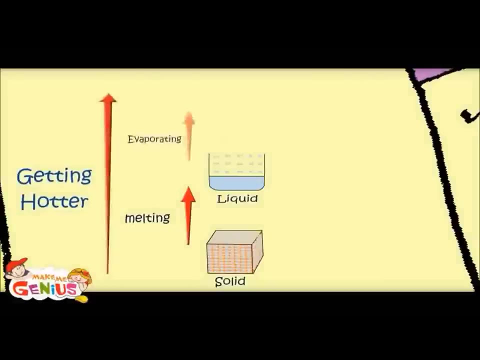 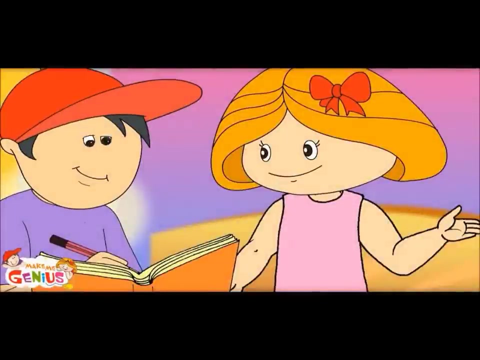 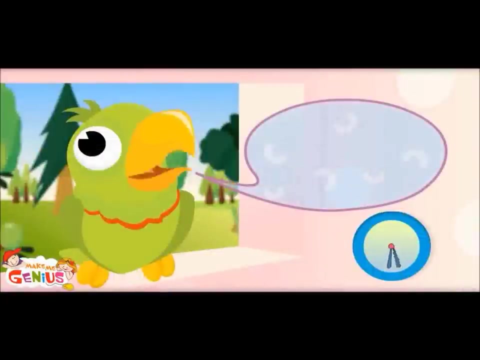 They come close to each other. It is called condensation. Very good, You are writing all: Wow, Jimmy, Do you know we can turn this liquid into solid? How? Just wait After some time. Oh, it has turned into solid again. 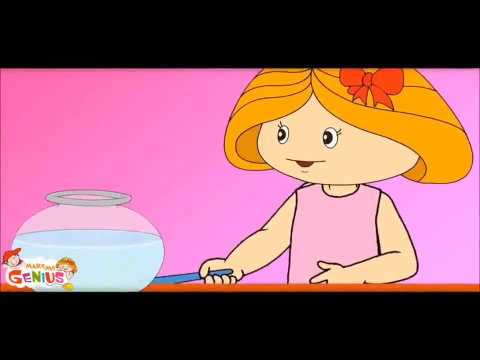 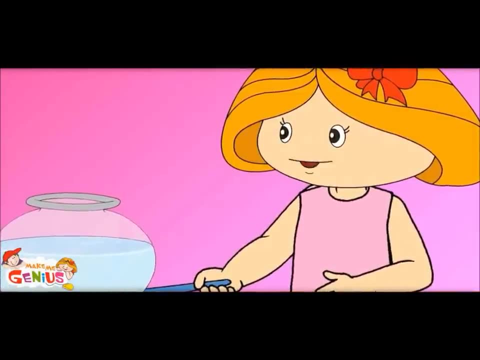 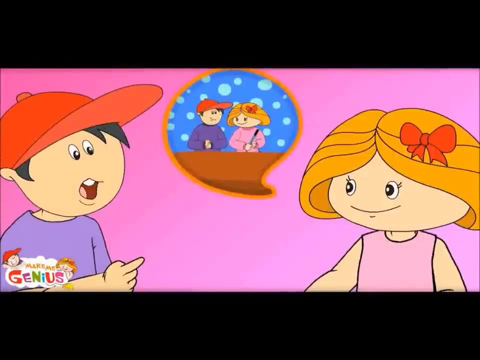 Yes, the molecules again become slow and come closer to each other And it becomes ice and solid. It is also called freezing. Oh, these molecules are like us in cold. We want to sit close to each other. Yes, you are right. 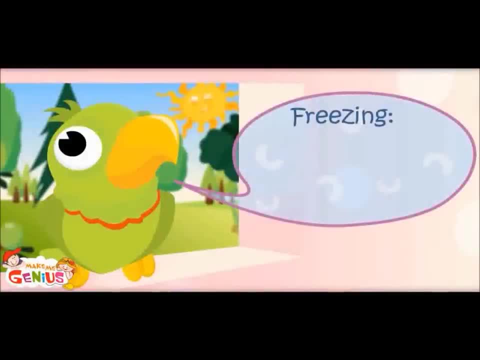 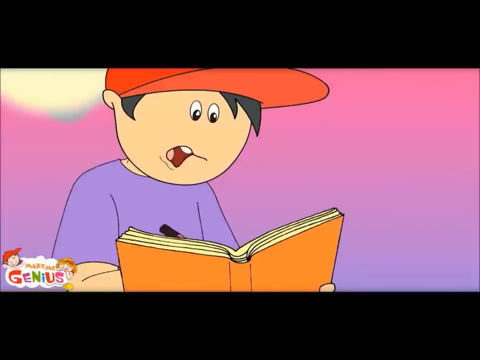 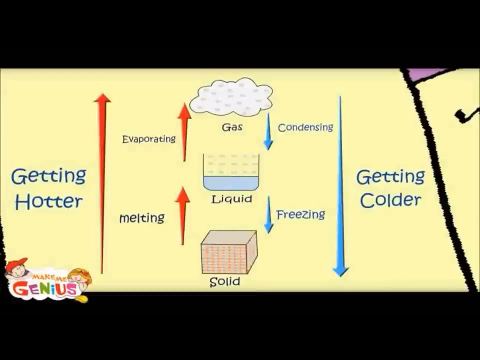 In summers we sit apart Freezing On cooling liquid, molecules come together and it becomes solid. Let me know, Tom, what happens to molecules when they are put in cold temperature. Thank you, Jimmy. Let me show you something. Oh, this grass is so wet in the morning. Yeah, there is lot of dewdrops on the grass. Dewdrops. How these are formed? It is condensation. Condensation, Yes, when air is full of water vapors and it touches the grass, which is cold, water vapor condenses and they forms water vapors.